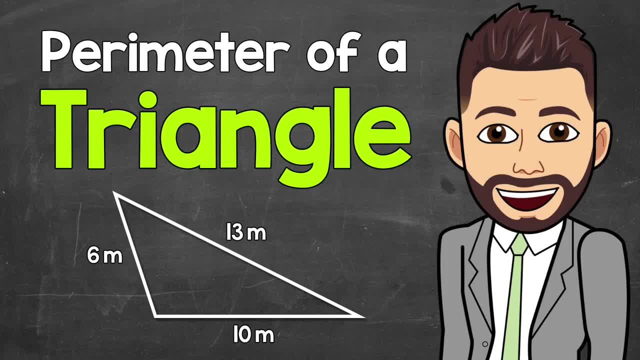 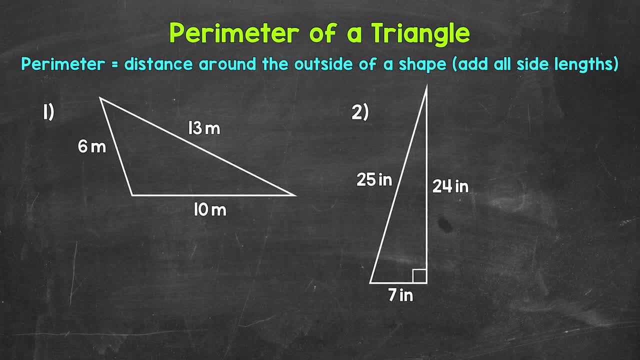 Welcome to Math with Mr J. In this video I'm going to cover how to find the perimeter of a triangle. Now, remember, perimeter is the distance around the outside of a shape. Let's jump into our examples, starting with number one. So let's find the perimeter, and we can do this by adding the. 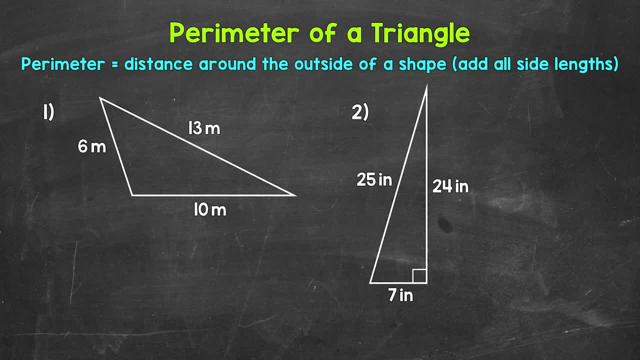 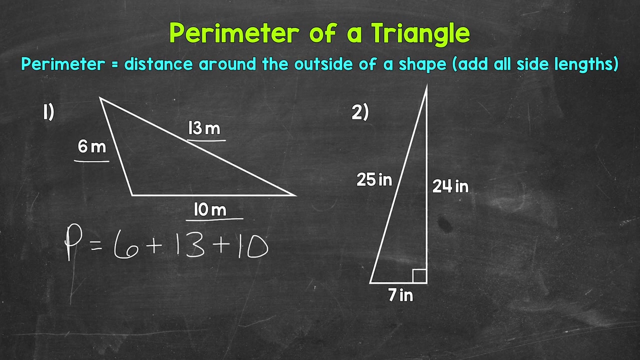 lengths of all of the sides, And since we're working with triangles, we will have three sides that we need to add. So perimeter equals. and then, as far as our sides, we have 6 meters, 13 meters and 10 meters, So 6 plus 13 plus 10.. Now it does not matter what order you add. 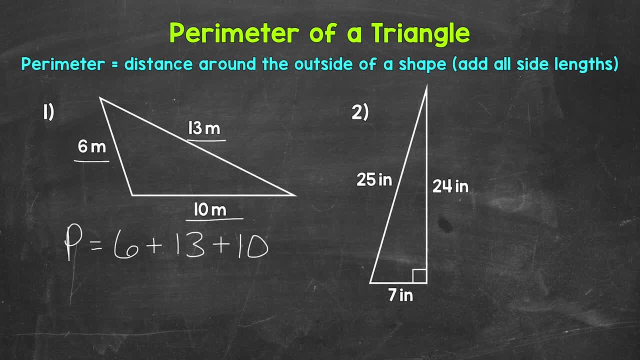 those sides in, You'll get the correct perimeter however you do it. So something to keep in mind. So now let's add: We have 6 plus 13,, which is 19,. plus 10 is 29.. So the perimeter is 29 meters. 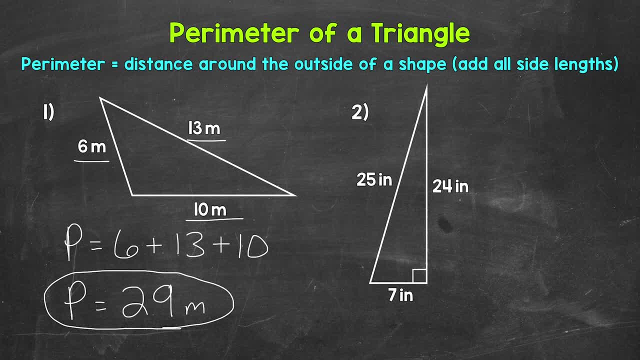 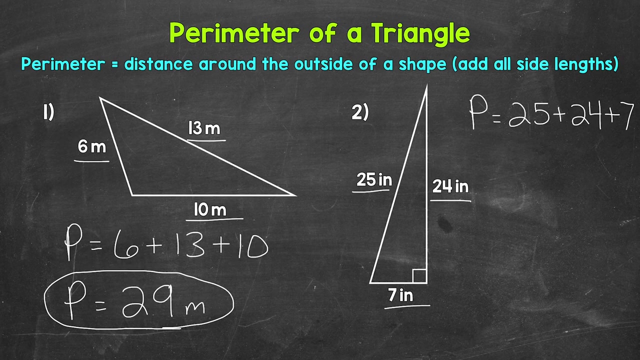 That means that the distance around the outside of that triangle is 29 meters. Let's move on to number two, where we have a right triangle with side lengths of 25 inches, 24 inches and 7 inches. So let's add all of these sides. Perimeter equals 25 plus 24 plus 7.. 25 plus 24 gives us 49 plus 7. 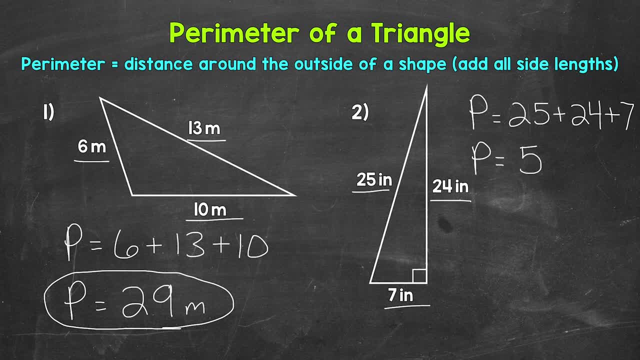 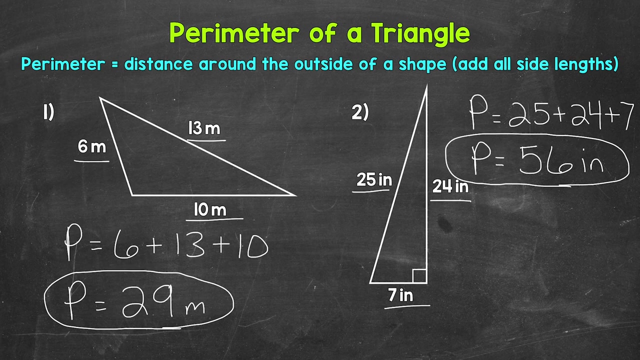 gives us 56.. So the perimeter is 56 inches. The distance around that triangle is 56 inches. So there you have it. There's how to find the perimeter of a triangle. Just remember, the perimeter is the distance around the outside of a shape and we can add all of the lengths of the. 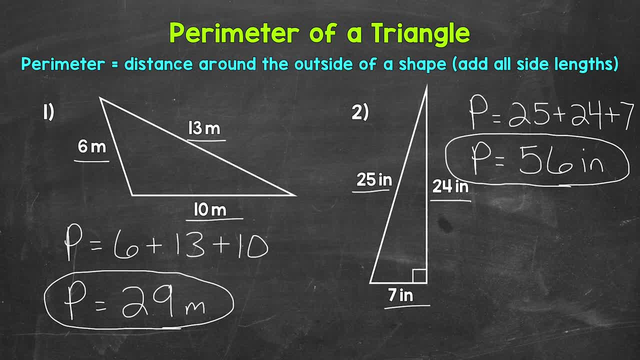 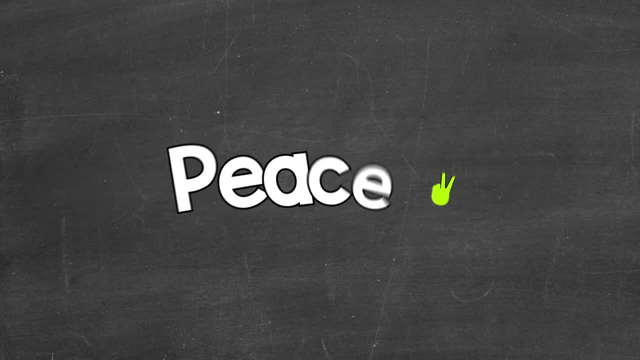 sides in order to find the perimeter. I hope that helped. Thanks so much for watching. Until next time, peace.